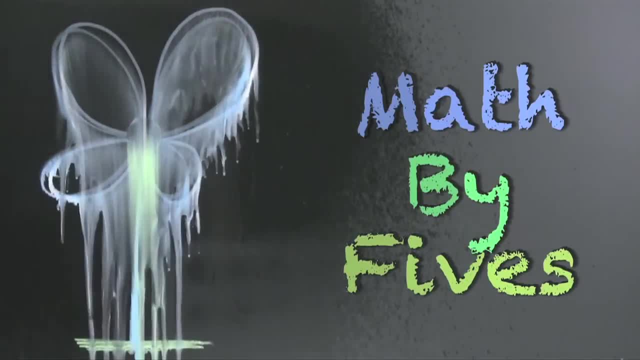 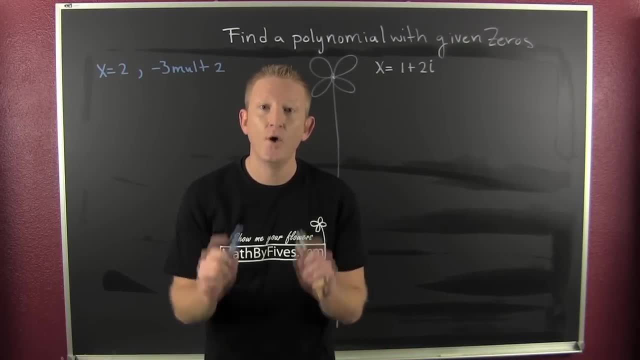 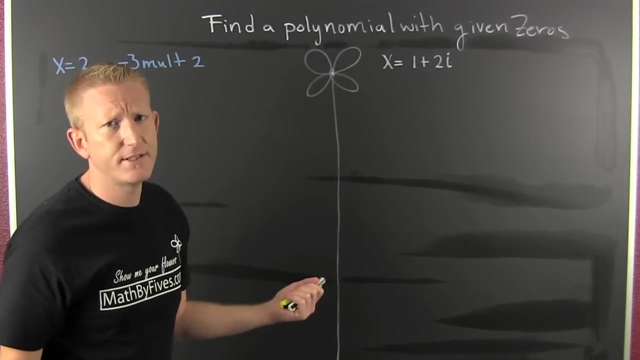 It smells like up-dogging here. The rock must be cooking again. What are we trying to do here? We're trying to find a polynomial with the given zeros of this degree of course. Okay, hey there people, This is kind of like the reverse of the zero factor property. Oh, 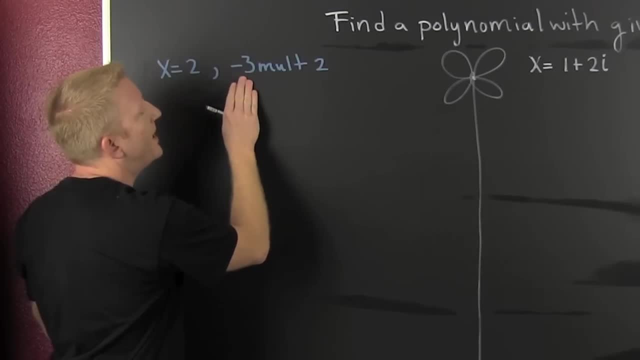 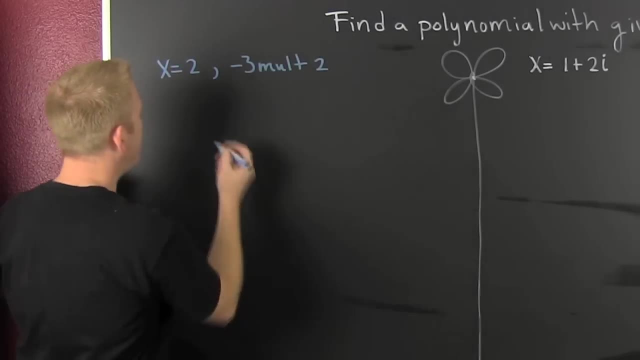 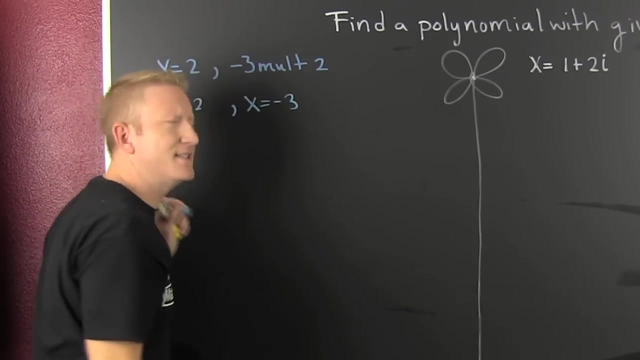 boy, I want this zero to be two and minus three with multiplicity two. What do you do? All right, let's just talk about what's happening here. This says that x is equal to two and x is equal to a minus three, But what is this multiplicity? bigger than one business That. 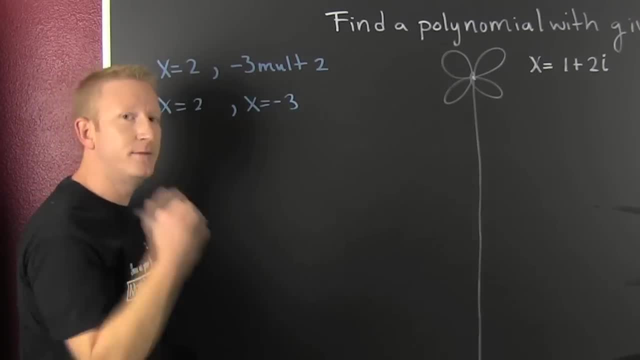 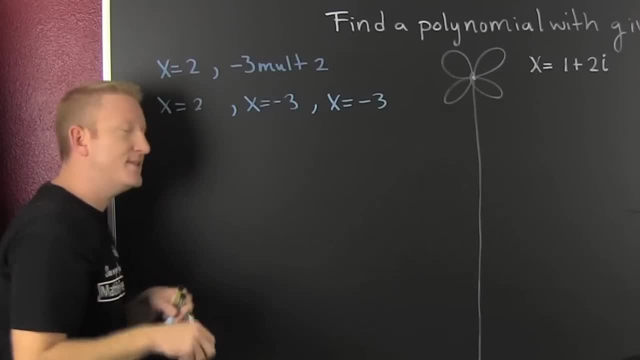 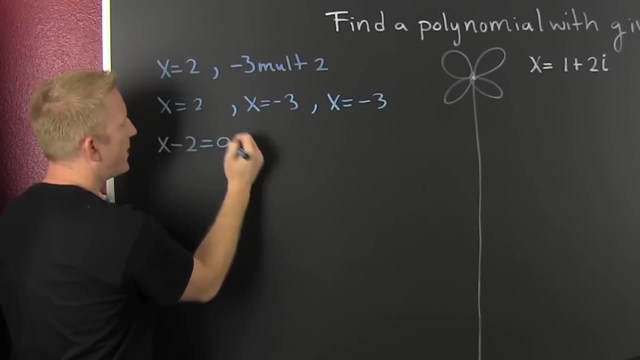 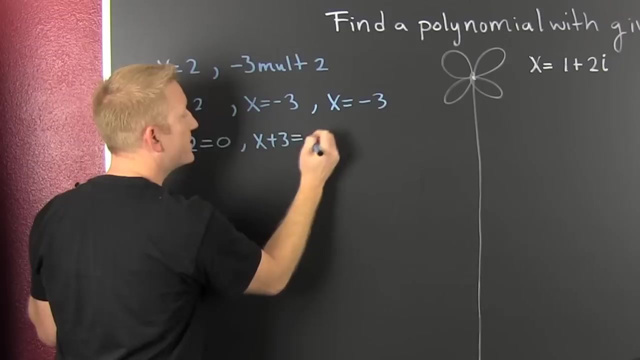 is equal to a minus 3, it happens twice Now. look what's happening here. Oh boy, If I subtract this 2 off each side, then I have x minus 2 is equal to 0.. And then if I add a 3 to both sides, I have x plus 3 is equal to 0. 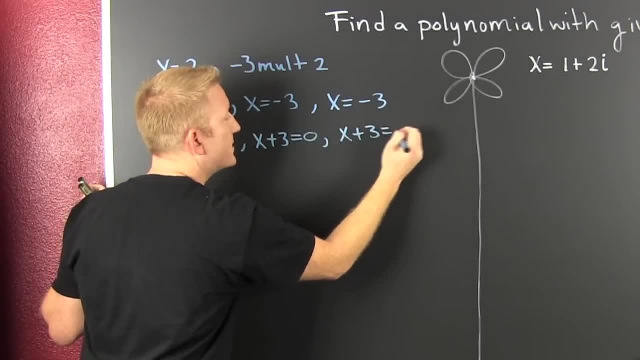 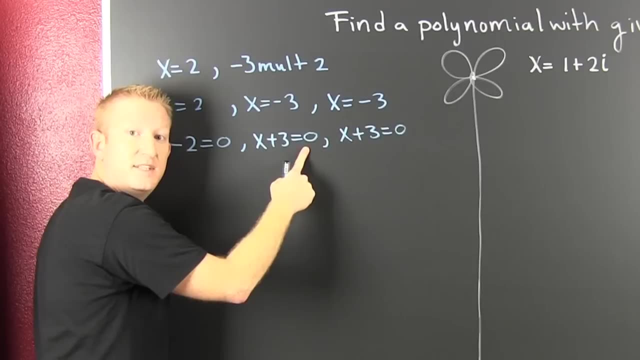 Okay, And further x plus 3 is equal to 0. Now if I take 0 and multiply it by 0, what's that going to be? 0!. And then if I multiply it by another 0? 0!. 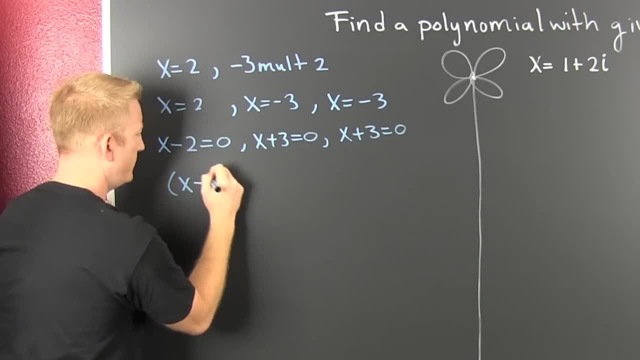 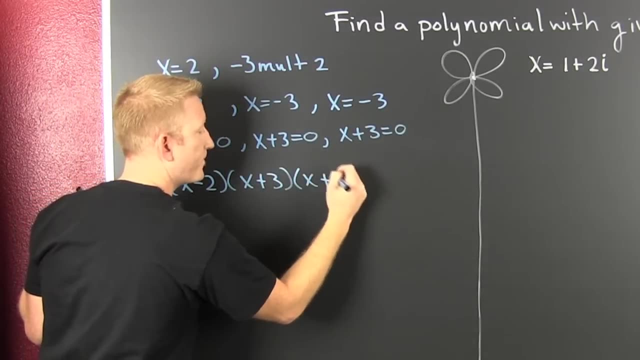 So we go and we multiply those two, We take this 0, and we multiply it by this 0, and we multiply it by this 0.. So if I take 0 times 0 times 0,, what do I have? 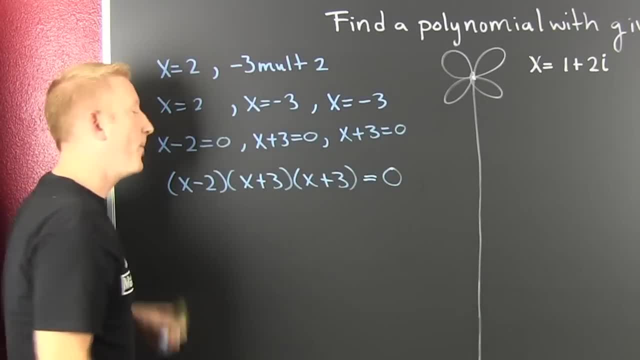 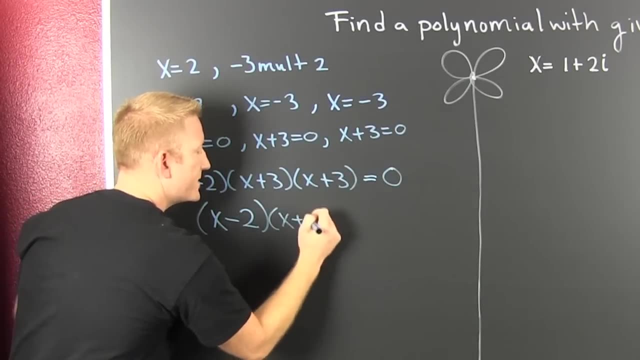 0.. For sure, for sure. Now you probably write it in a little more compact notation. and then you say that this is x minus 2.. x minus 2 times x plus 3 squared, That's equal to 0.. Now I realize, after you do this a few times, you're going to jump. 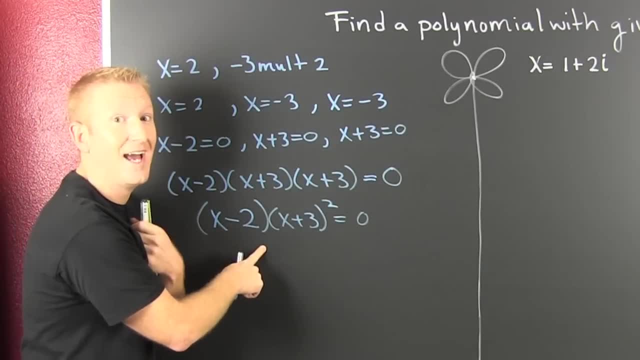 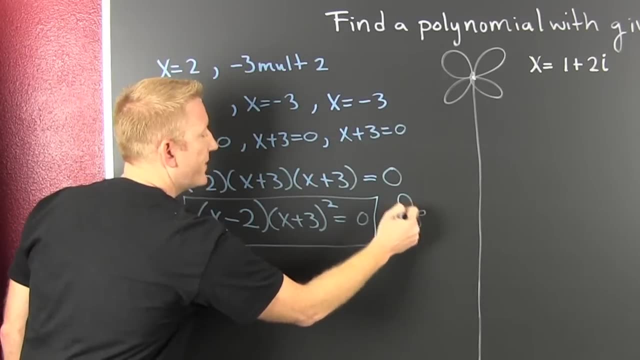 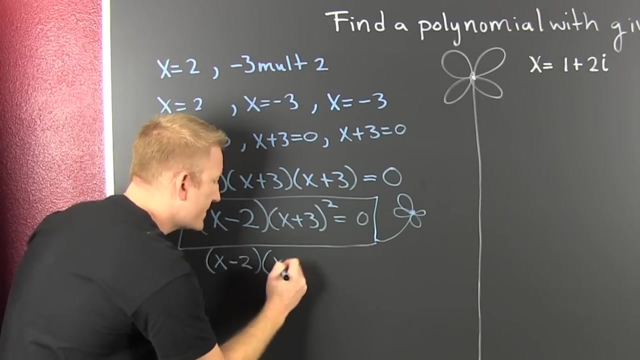 from here to there, And that's fine. I don't mind Bucks and flour. But perhaps you want to multiply that out. You're all like x minus 2 times x squared, this one times that one double it plus 6x squared. 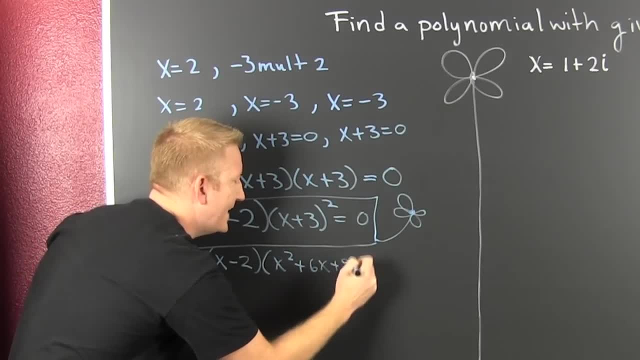 x squared this one times that one double it plus 6x squared 6x plus 9.. Fine, That's still equal to 0. So then you go, and you go a little bit further, and then you multiply all these guys out. 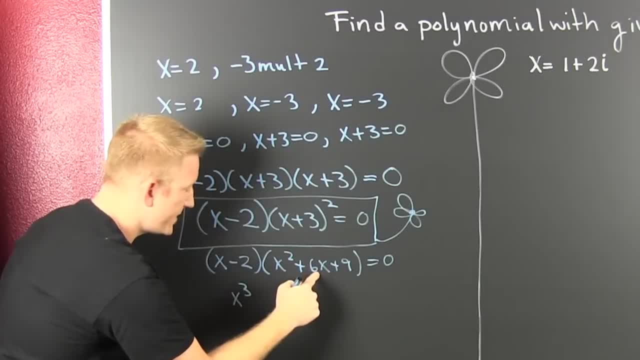 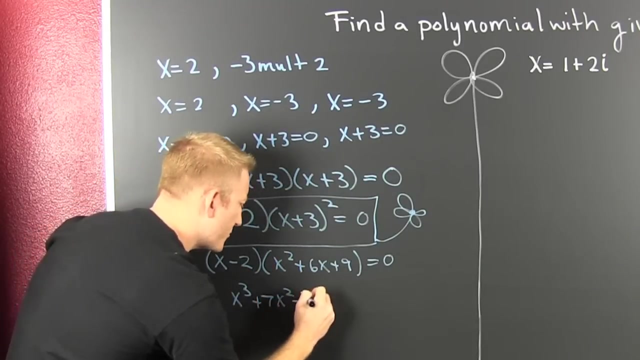 and you find that this is x to the third. Then there's a 6x squared plus an x squared is 7x squared, And then x times 9,, that's 9x, And then 9x minus 12x is minus 3x. What's next? 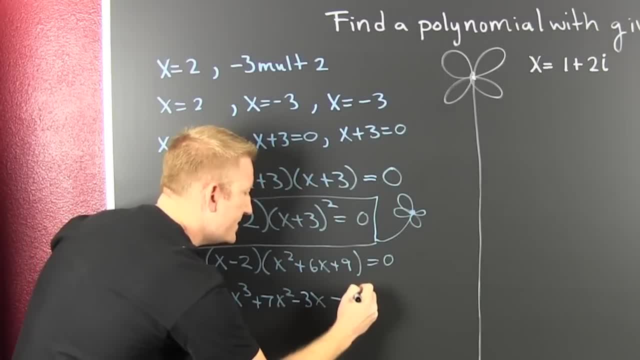 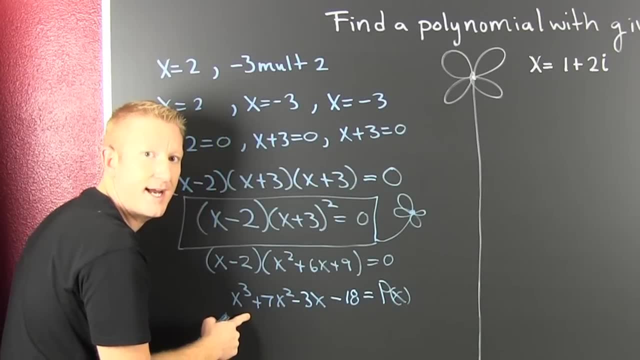 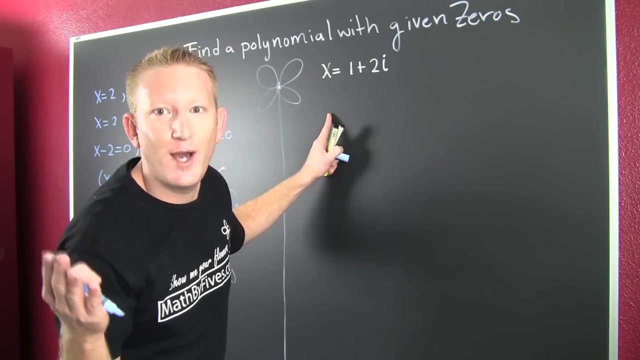 That last term, Oh, minus 18, and then this is going to be a polynomial. Now, if I didn't multiply that out, right, make sure you put it in the comments down below. Let's go over to here. This one's more complex. 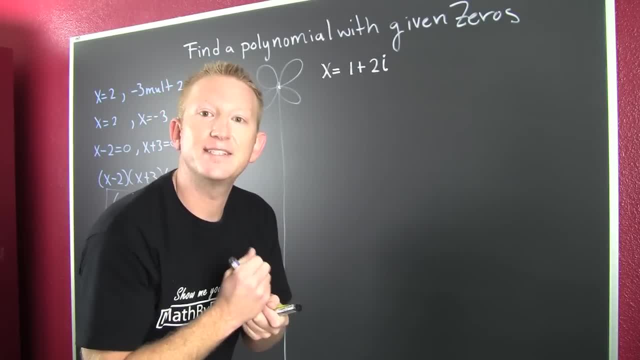 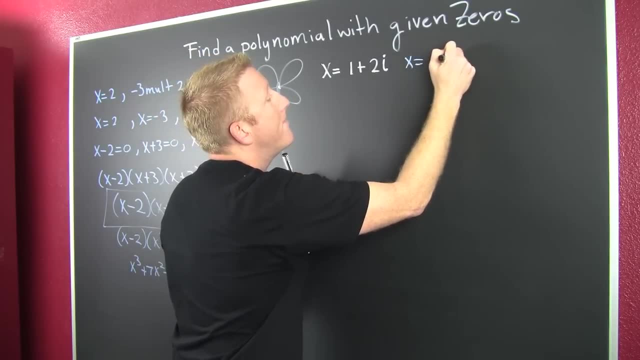 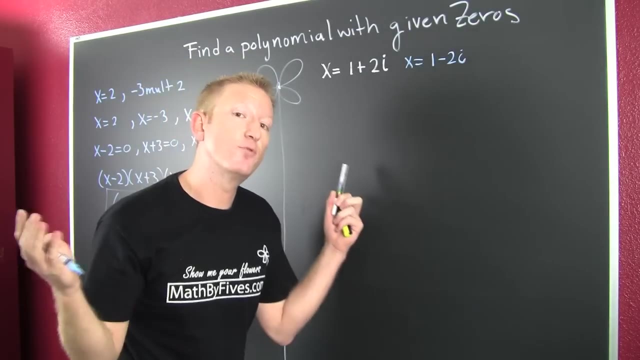 You have a complex zero. Hoho, Complex zeros theorem. They happen in conjugate pairs. That also means that x is equal to 1 minus 2iy. That's perfect, Awesome, Cool, Because this is a zero. so in order for the polynomial to have real coefficients, you 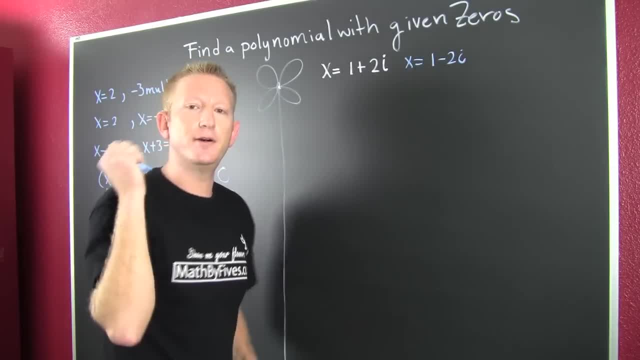 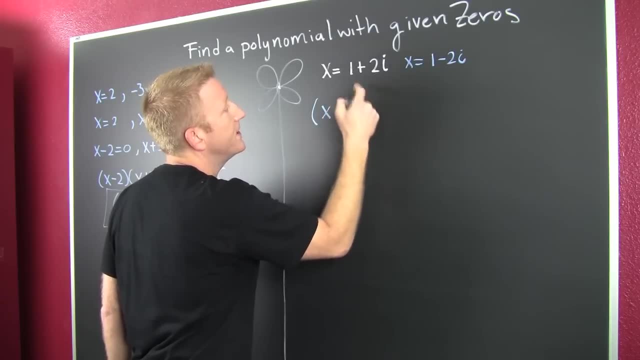 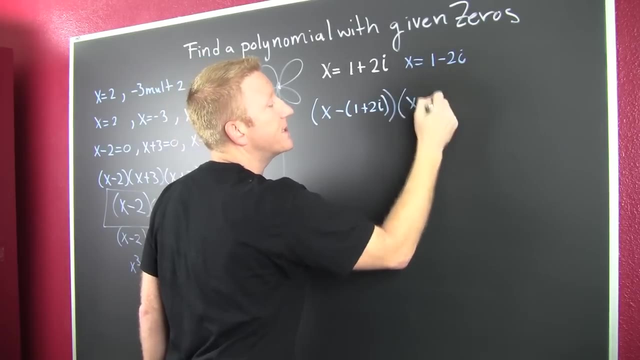 need to have the conjugate in there so that when you multiply them out it has real coefficients. Let's go So. this is x minus this guy, 1 plus 2i times x minus this guy, 1 minus 2i. 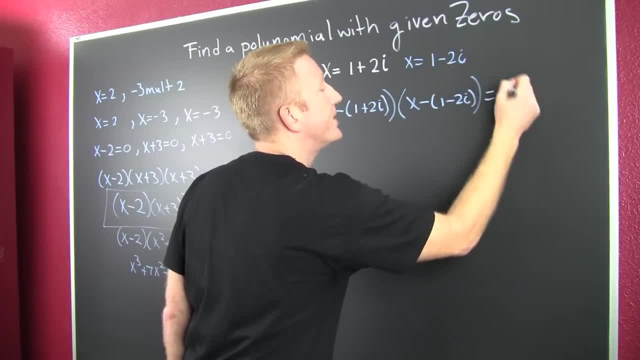 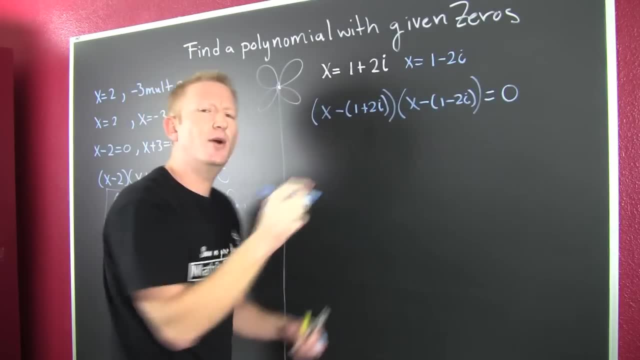 I'm stepping skips here, Like over there. we said, you probably just jump here, Alright, so it's x minus the zero. that's the factor. Let's go ahead and multiply this out so that we can find that polynomial really does have. 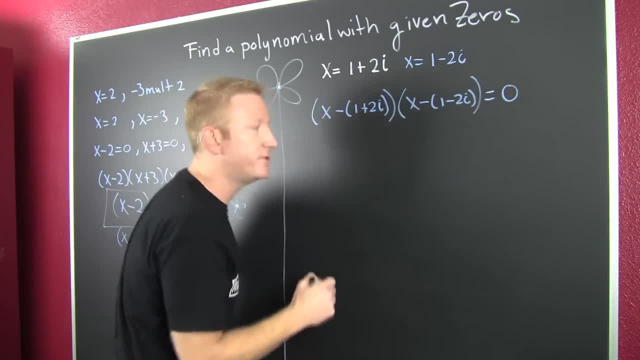 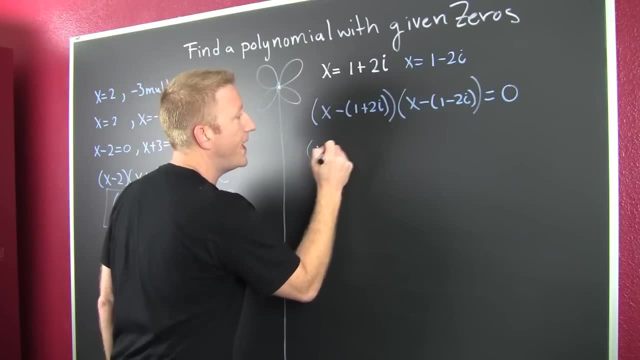 real coefficients. So then, here's what I recommend you do. This is tricks. It's like ollie kick flips, You're like whoa Yeah. so we go. We call it: x minus 1 minus 2i.